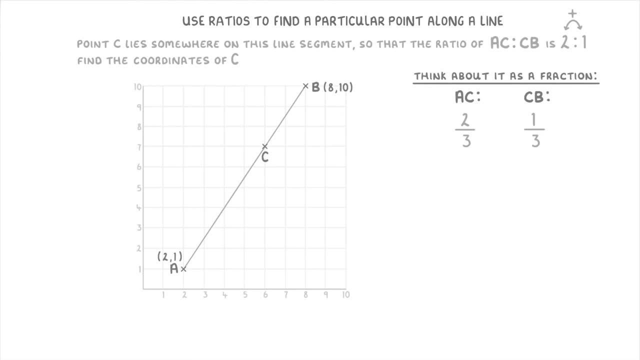 and y axes. For example, the x values change from 2 at A to 8 at B, so that's a change of 6.. While the y values change from 2 at A to 8 at B, so that's a change of 6.. While the 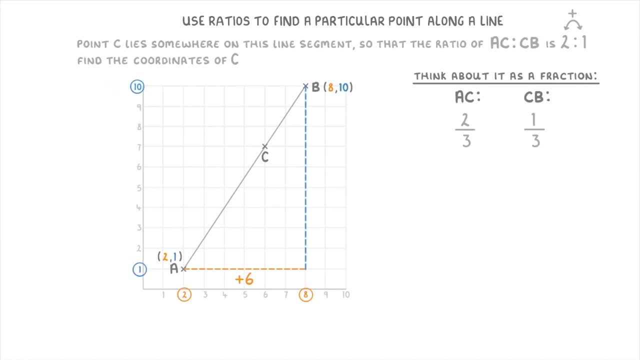 y values change from 1 at A to 10 at B, so that's a change of 9 in the y direction. Then, because we know that C is 2 thirds of the way between A and B, we just need to find: 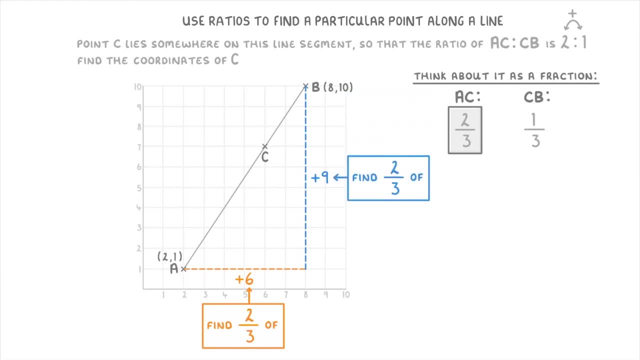 2 thirds of the change in x and 2 thirds of the change in y, because that will tell us how far we need to move along the x axis and up the y axis to get from A to C. So for the x axis we're to do 2 thirds of 6, which is 4, and for the y axis we're to do 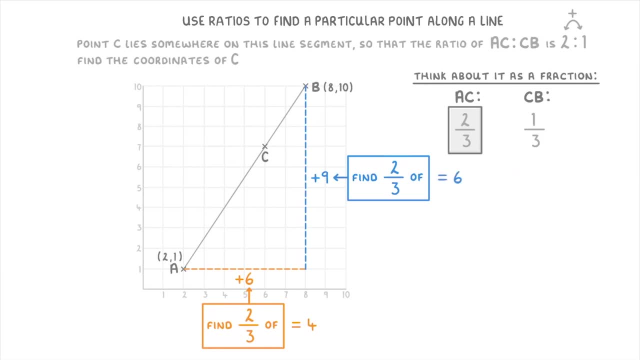 2 thirds of 9,, which is 6.. Then all we're going to have to do is add these values to our point A coordinates, and that should give us the coordinates of C. So if we add 4 to A's x coordinate of 2, that will give us 6 as the x coordinate of C, and if we add 6, 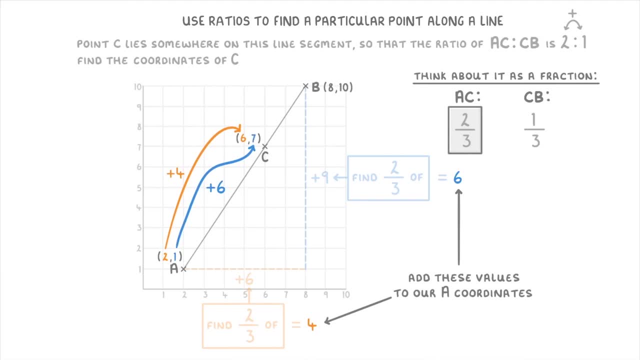 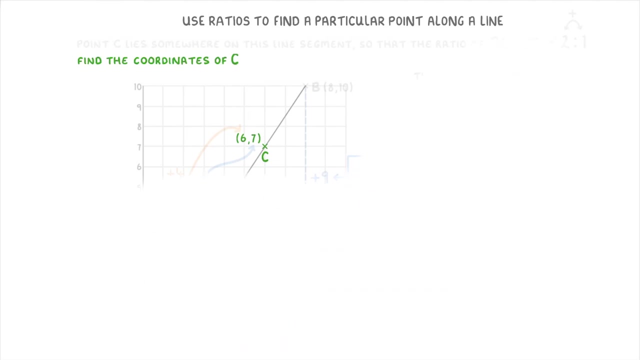 to a's y-coordinate of 1, that will give us 7 as the y-coordinate of c, And that's it. We've now found that c is at, which is 2 thirds of the way between a and b. Let's try an exam-style question this time. So this question says that points a and b 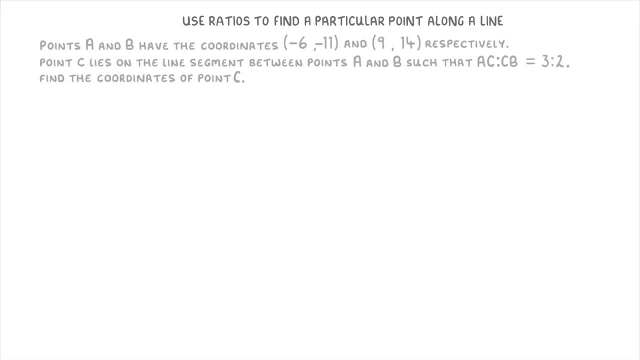 have the coordinates and respectively: Point c lies on the line segment between points a and b, such that a, c to c, b is 3 to 2.. Find the coordinates of point c Now for questions like this, if they don't give you a graph as part of the question. 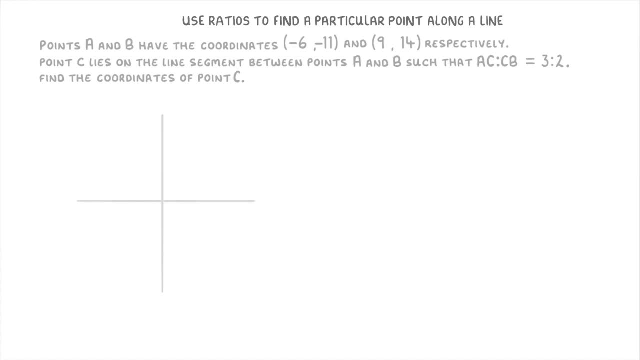 it's normally going to be a lot easier if you just sketch one out quickly And because it's just for your own benefit, you don't have to worry about it being perfect. For example, you might not even put numbers on the axes, You just put your two points. 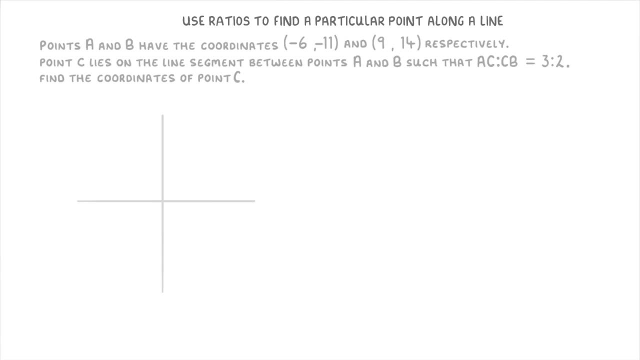 roughly where you think they should be. So for this question we can start by putting point a down here at roughly, where we think negative 6 and negative 11 should be, and b up here at And if you put it somewhere, 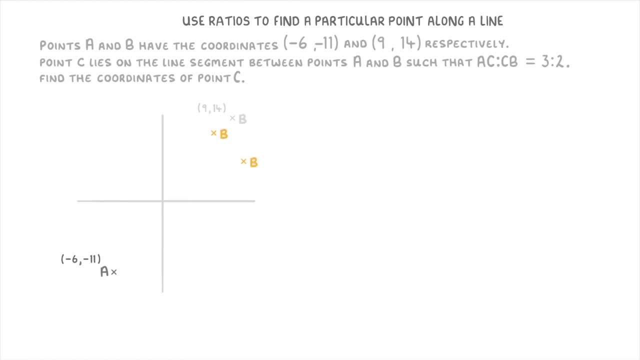 slightly different, like down here or over here, it really doesn't matter, It won't affect our working out at all. Next, you want to draw your line segment between A and B and put point C roughly where you think it might be. And again, it doesn't matter if you don't put it in exactly the 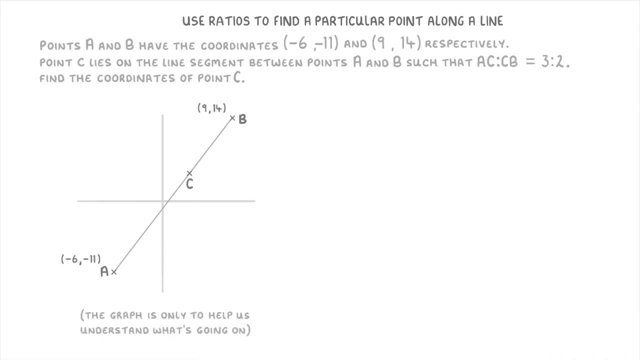 right place. The graph is only to help you understand what's going on in the question Next up. we know that the ratio between these two parts is 3 to 2.. And remember that means that this part is 3 fifths of the line and this part is 2 fifths. 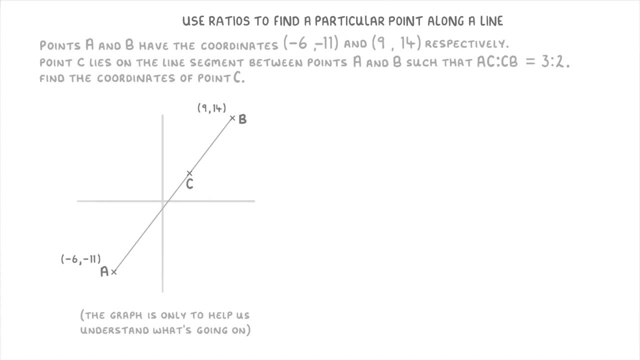 To be clear at this point, all we've done is take the information from the question and sketch it out onto a graph so that we can more easily understand what's going on. To actually answer the question, though, and find C. 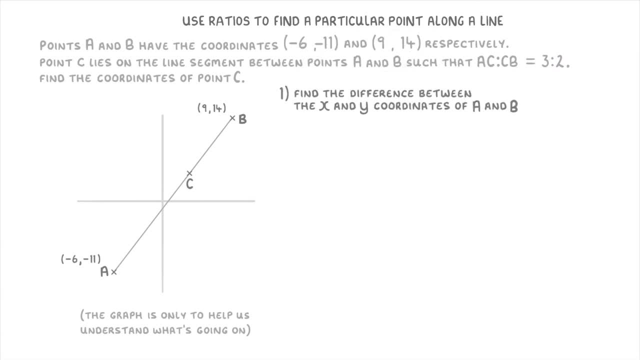 we need to do three things: First, we need to find the difference between the x and y coordinates of point A and point B, So the change in x and the change in y. Then, second, we need to find 3 fifths of that difference. And finally, third, we need to add that 3 fifths. 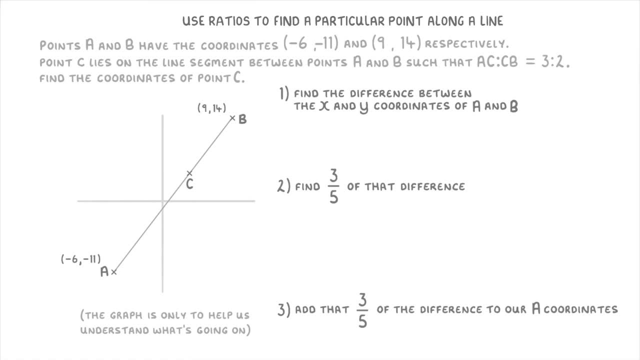 of the difference onto our A coordinates. So for step one, the difference between negative 6 and positive 6 is 1.. And the difference between negative 6 and positive 6 is 1.. And the difference between negative 6 and positive 9 is 15.. So the change in x is 15.. While the 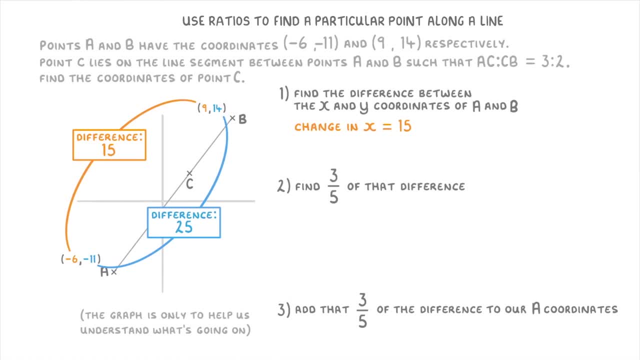 difference between negative 11 and positive 14 is 25.. So the change in y is 25.. Then for step two, 3 fifths of 15 is 9.. And 3 fifths of 25 is 15.. And then finally, for 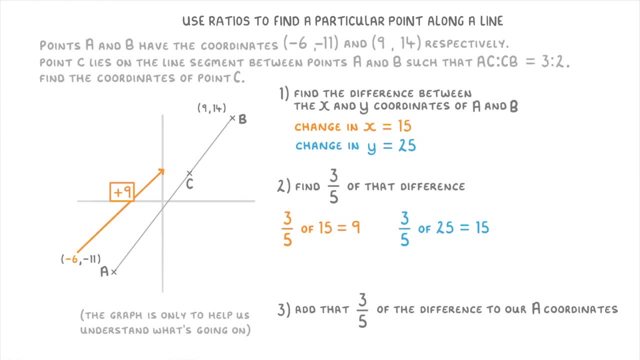 step three: we need to add 9 to A's x coordinate of point B. So we need to add 9 to A's x coordinate of negative 6, to find that C's x coordinate is positive. 3. And add 15 to A's y coordinate of negative 11, to find that C's y coordinate. 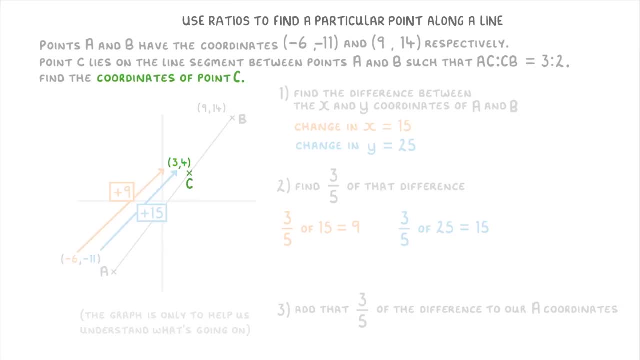 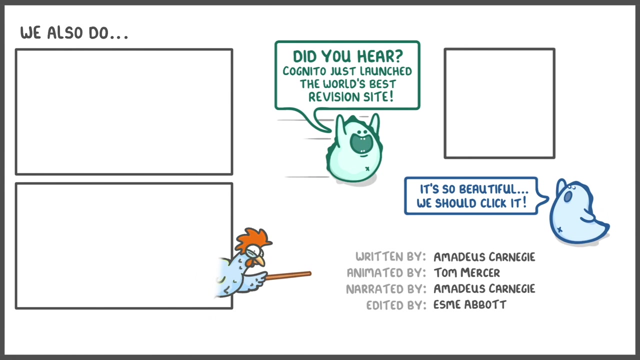 is positive 4. And that's it. We've now found that C's coordinate is 3, 4.. That's it for this video, So hope you enjoyed it and cheers for watching. Subtitles by the Amaraorg community. 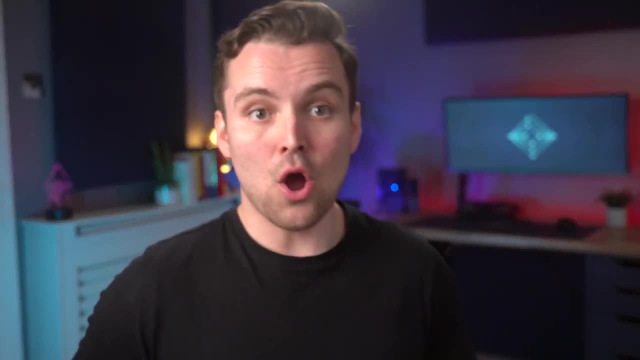 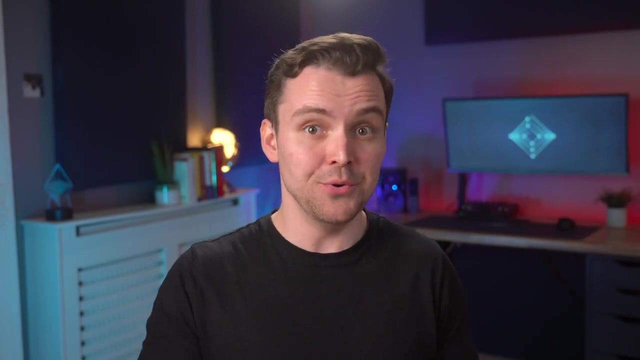 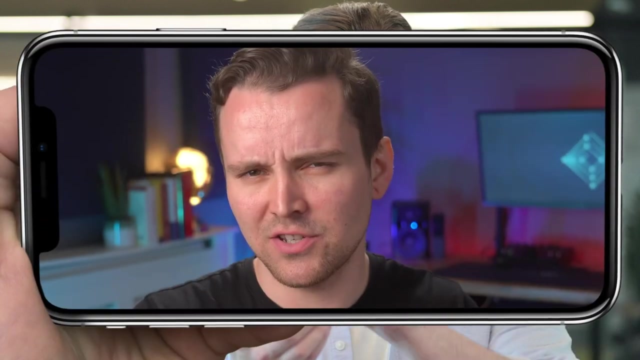 Oh, you've just found me bonding with my Firefox Web browsers. Web browsers- Who needs them and who wants them? Well, you need them, And if you're watching this video, then you probably want at least one. The most used program on pretty much any device is its web browser, which is no surprise, since 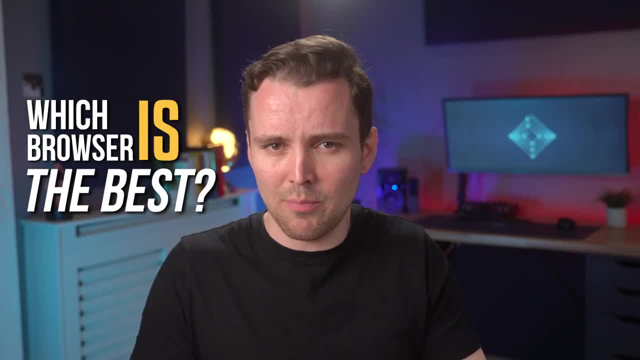 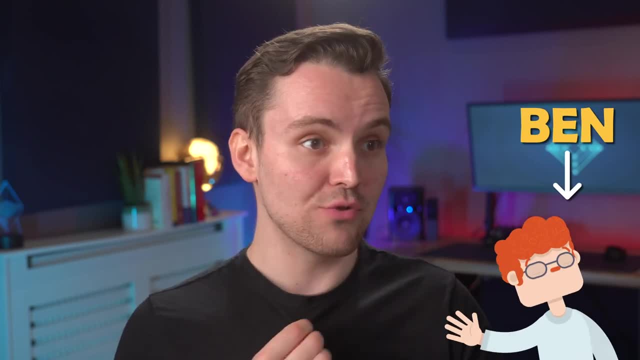 none of us would know how to function without the internet. But which browser is the best And which should you be using? I'll answer these questions and more throughout this video. Now, my editor, Ben, has been asking me to wear a green shirt on screen for a while now. 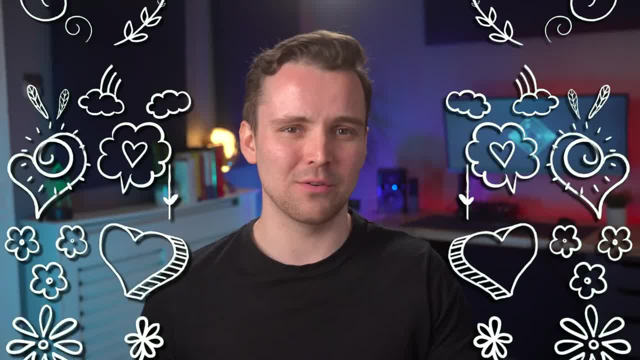 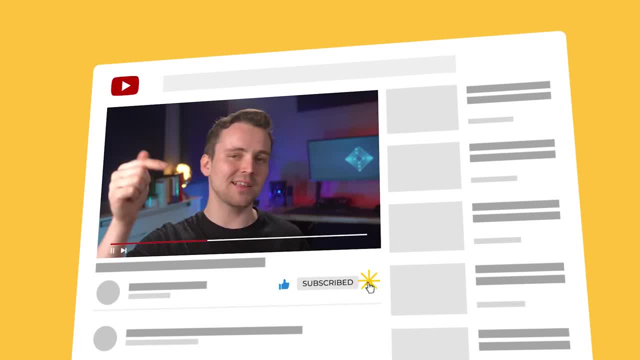 Now we all know what that means. He's going to edit some really weird stuff onto it. I told him I'll only do it if this video gets to 5,000 likes. So have at it, my little friends. Press that like button and subscribe. 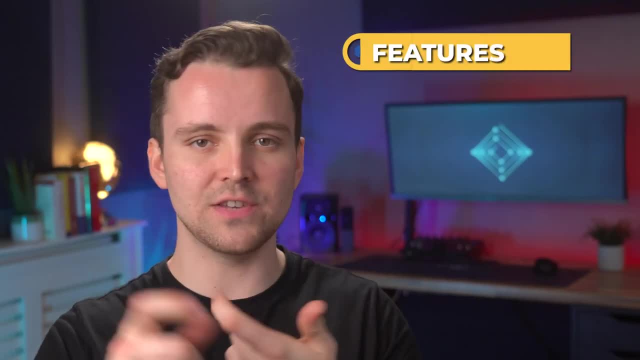 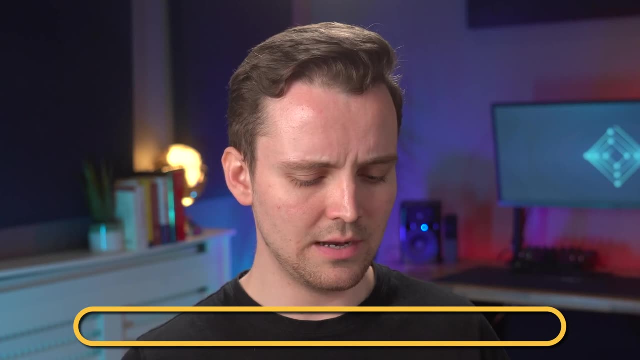 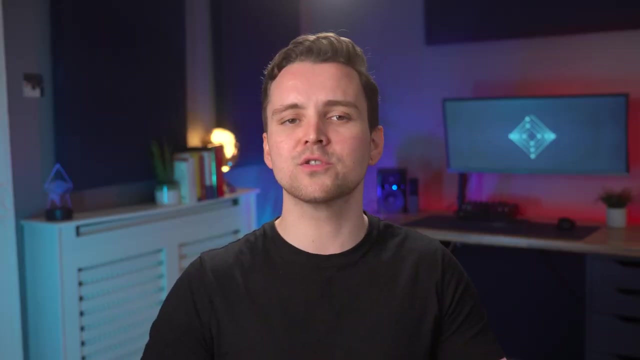 Now I'll be reviewing each browser based on the same criteria: Its features, its availability, whether it's free or not, and how much the company knows about you based on your weird searches. Can you eat yogurt that expired two years ago? Starting us off is Google Chrome. Google Chrome is by far the most popular web browser. 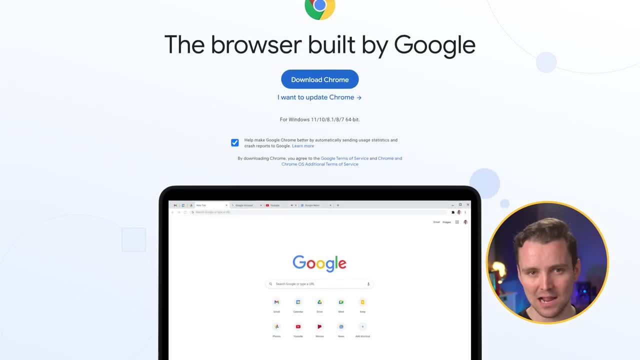 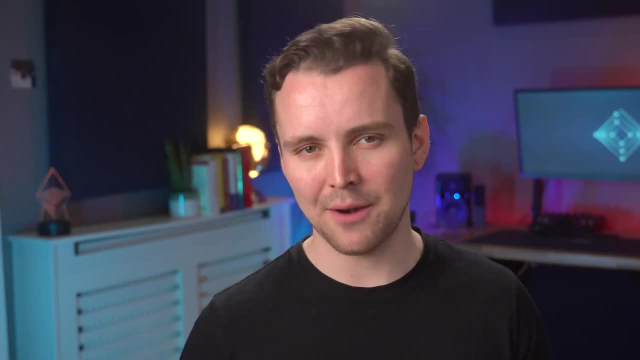 in the world. You're probably watching this video from a Chrome tab right now, squished in between the 16 other tabs that you've had open for weeks. The free-to-use browser's popularity is mainly due to its cross-platform compatibility. wide 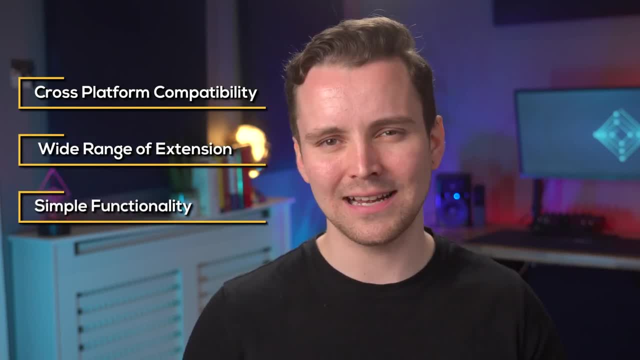 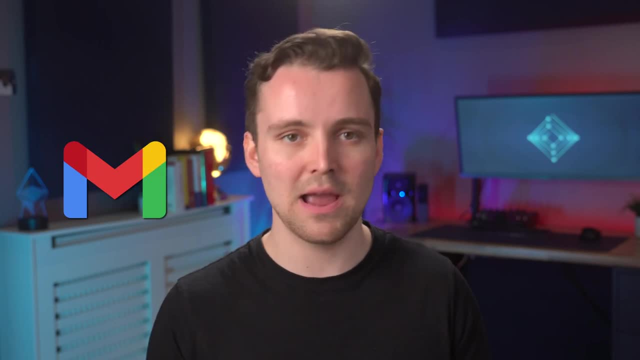